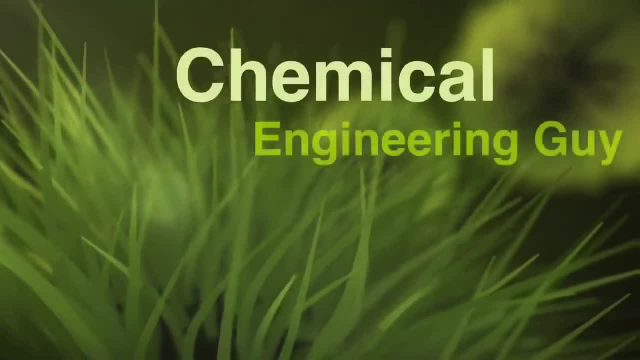 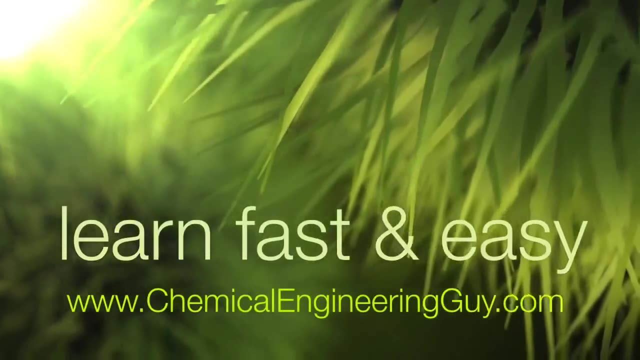 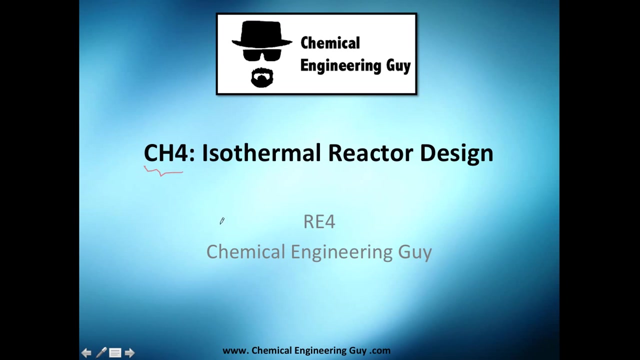 Guys, we're going to start chapter number four, which is isothermal reactor design, and things are going to get way more interesting because we are going to actually start developing what we've seen before in chapter one, chapter two and chapter three: we're going to apply it for our reactors and 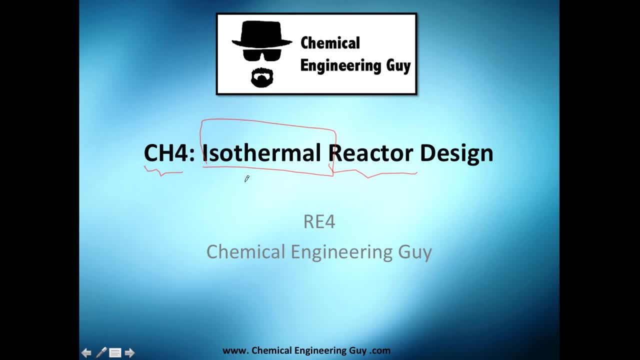 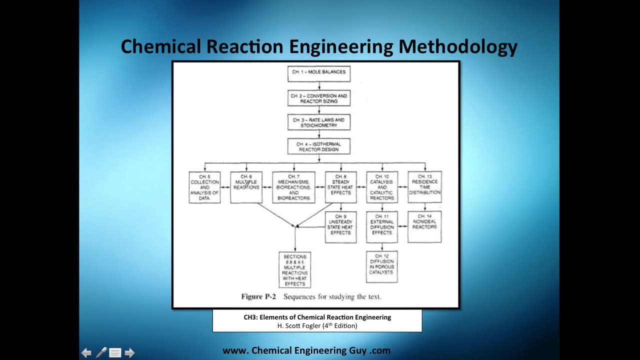 especially in isothermal design. What does that mean? That means that we have no temperature changes, so we have no Q or etc. We are not going to take care on that. we're going to suppose temperatures are the same. So, as usual, I'm going to show you this diagram. we've seen chapter number. 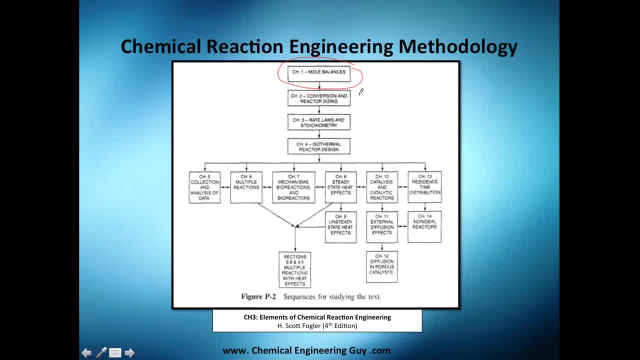 one which is model balances or design equations. then we saw a little bit of conversion and retro sizing, essentially CSTR and PFR, given a rate of reaction versus conversion, Let's say a table. they give you the data and it was fine. you could use this data directly and you didn't need to get 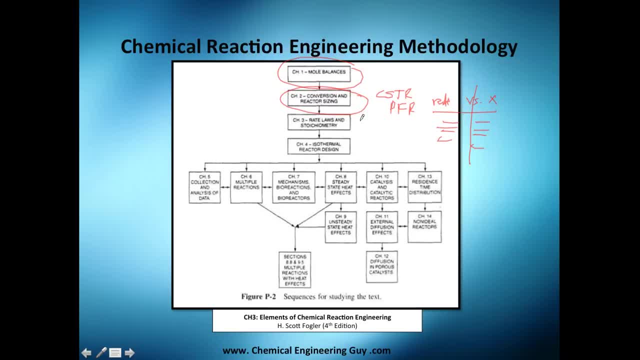 a rate law, Then after that we have the reaction, and then we have the reaction, and then we have the reaction, and then we saw some theory about chemistry or chemical kinetics, the rate law and some stoichiometry tables. I think the part of stoichiometry tables is kind of boring, but we need that for our 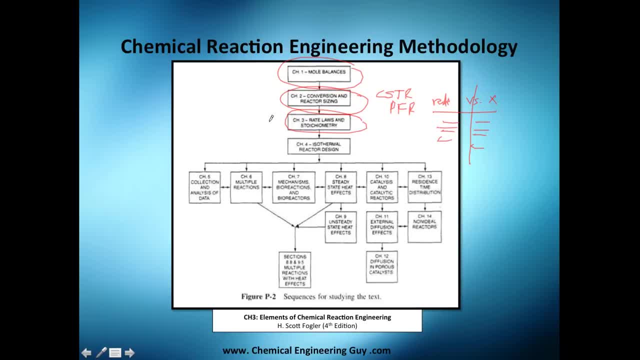 let's say, mathematical procedures. And finally we are here chapter number four, which is isothermal reactor design. So, as you see, after you finish this chapter, you will have the essentials on the reactor engineering. Now, what does that mean? It means that after that we're going to follow. 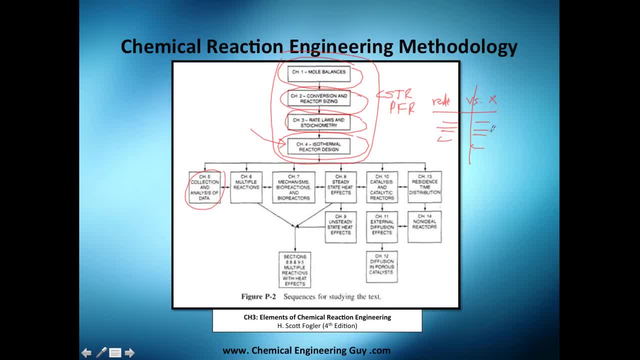 chapter 5, which is collection and analysis of data, which is essentially getting this information and apply it to a rate law. We're going to focus more in the rate law and rather than the reactor per se. And then you continue with chapter 6, which is multiple reaction. That's one important thing. 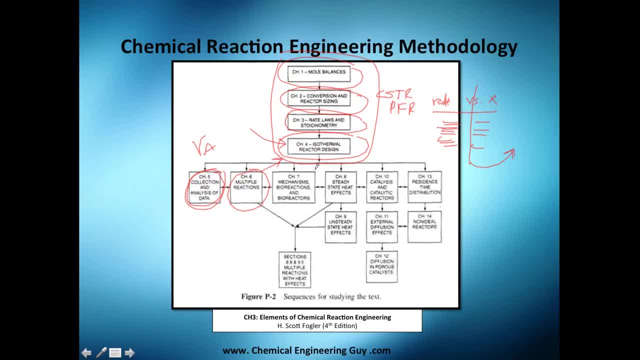 I want to tell you guys, We are just seeing some data on the reaction process, also now from this isothermal reactor designed with one reaction, which is very normal. don't think it's useless. actually, many processes involve only one reaction, but of course you know there are sometimes you have multiple reactions. then we see. 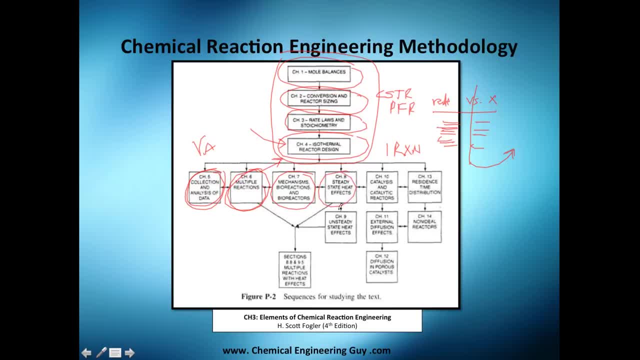 a little bit: mechanical reaction, steady-state heat, etc. so all these are, let's say, just an overview of the topic and this chapter here, chapter 8, steady state heat effects is when you have non-isothermal reactors, so when the temperatures are not the same. so right now, just focus that we have same. 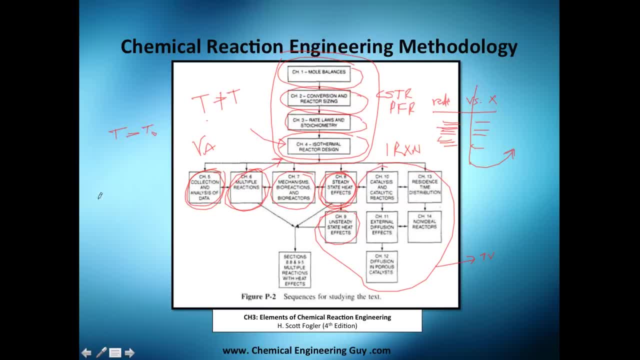 temperature, not temperature change. we will have pressure drops. so yes, we will maybe have pressure changes and of course in gas phase we're going to have volume changes. we've seen that before in rate law and stock character, so hopefully you have a good idea of what we're going to talk about in the next chapter. 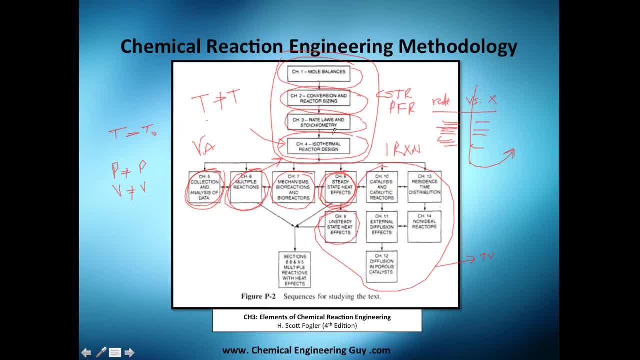 you are interested in the topic because it, I think, is one of the most interesting ones. maybe mole balance is very nice but you don't get to use those equations that much. and converting and reactor sizing is a good chapter because you get to know how to size the reactors rate law. maybe it's kind of boring if. 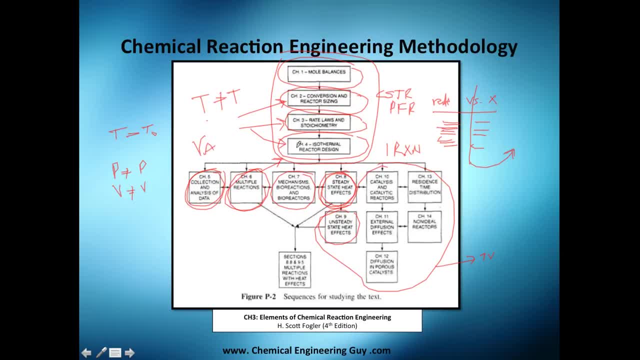 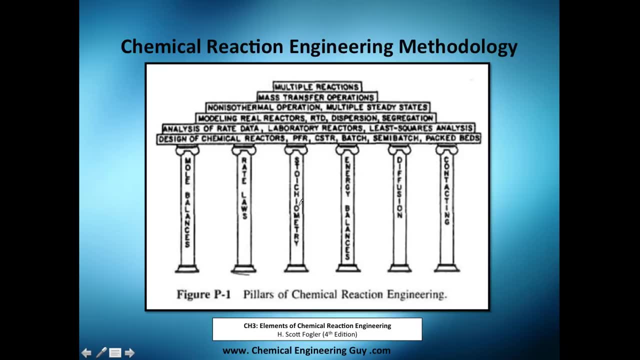 you don't like chemistry. if you do like it, it's nice. but now, right now, if you love engineering, you're going to love this chapter. so, once again, this pillars which in this one- chapter 1, chapter 3- and we still don't see these guys here. but what you're going to see is that we can essentially start with. 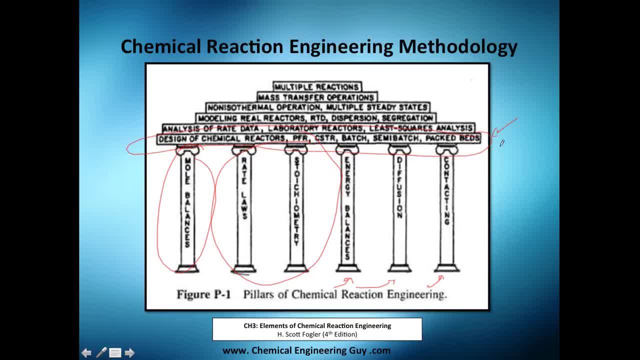 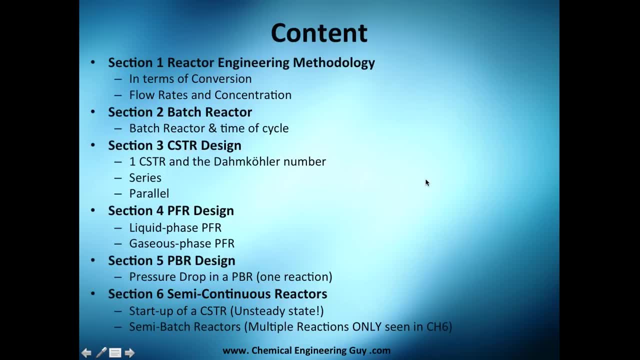 our first step, which is the sign of chemical reactors such as PFR, CSTR, batch, semi batch and pack pets. actually, let me show you the content of this chapter, chapter number 4, I just broke it. in section 1, which is rector, engineering methodology, we're 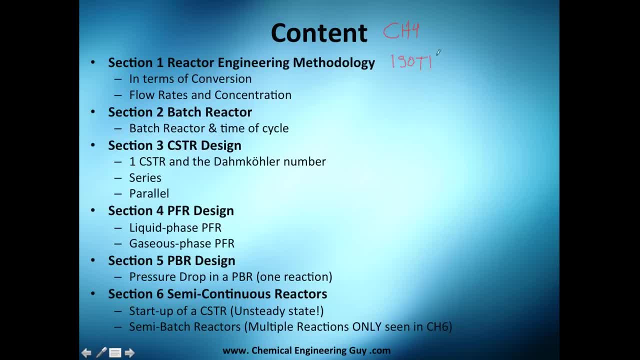 going to see how to, or isothermal reactors, of course, how to account for, let's say, a PBR or a PFR CSTR, when is convenient to use a conversion and when is convenient to use flow rates or even concentration. I think concentration is always a goal. so if you have problems that you have no idea, just 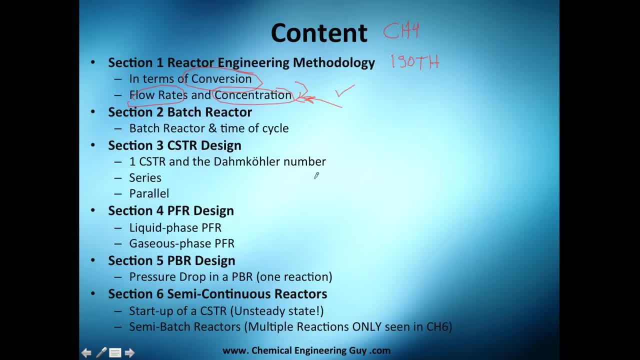 go with concentration and you will be ok. of course, you will need to use the laureate biometric tables now, while we see that it's a little bit theory, doesn't worry, it's not that much. then we keep going with our batch reactor analysis. I know we've seen some. 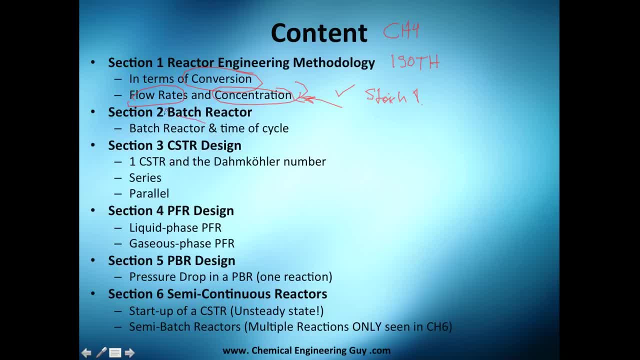 exercises before, but we're going to do a little bit more, especially first order and second order reactions. then we see the stoping, which is time cycle, is very, very simple but it's important to take care of it. Then we continue to section three, which is CSTR, or continuous-tiered tank reactor design. We start with the first. 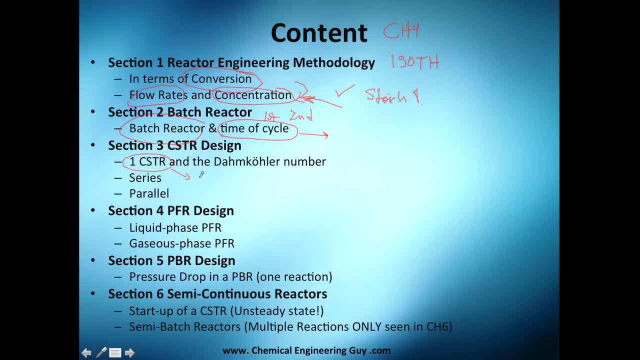 we've seen a lot of the first we're going to see first, but only one reactor first. differential of first rate, sorry, first rate of first order rate and second order rate, And we use this number here. we're going to introduce it. it's cool, it's going to help us a lot to understand the reaction or the 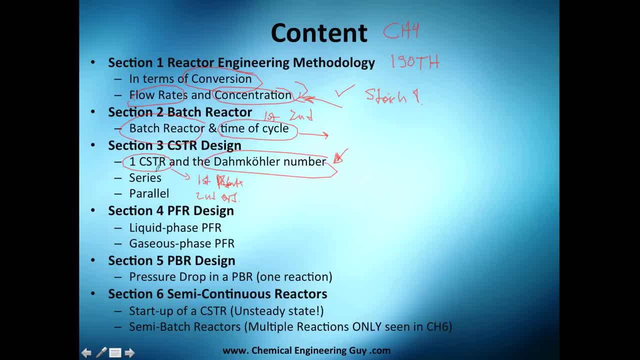 conversion rate is the Damkohler number. Then we keep with series CSTRs and parallel CSTRs, which probably you're thinking that we saw this in chapter two. that's true, but now we're applying this first order, second order, zero order, rate of reactions. Then we continue with section four. so by now you should. 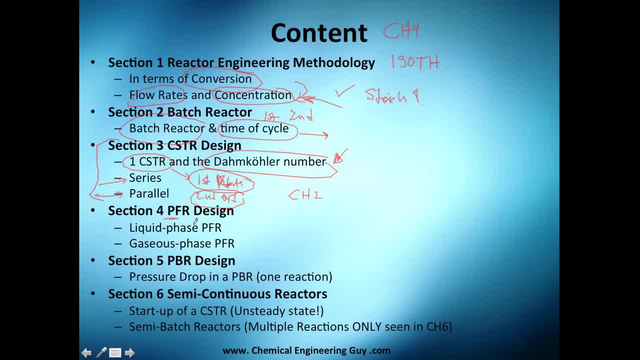 know a lot of CSTR and batch reactors. then we continue with PFR, which is plug flow reactor. We see liquid phase and then we see gaseous phase. Liquid phase: you know it's easy, because volumes are the same. Gaseous phase: in general you don't have volumes you actually need to account for. 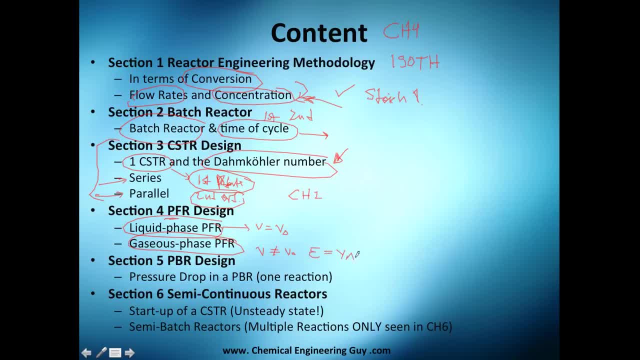 the change in moles and all that stuff. Hopefully you remember that from our previous chapter. all these dichrometric tables. I'm not going to explain how I use these tables, I'm just going to use them. Maybe I tell you that it's for. 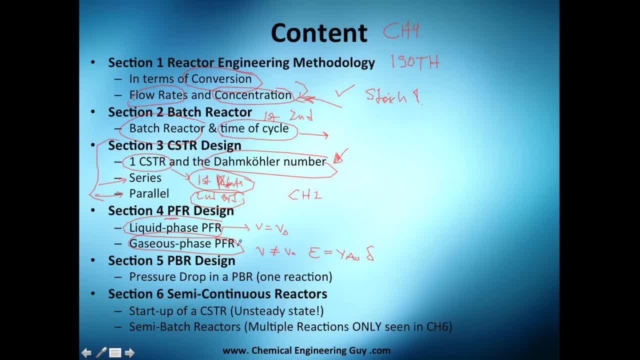 example for a gaseous phase, PFR. If you have no idea of what I'm talking about, I recommend you to go to chapter three and read again, make a review and then maybe you can see what I'm talking about. You can get the topics here. Anyways, then we continue with PBR, which is packed. 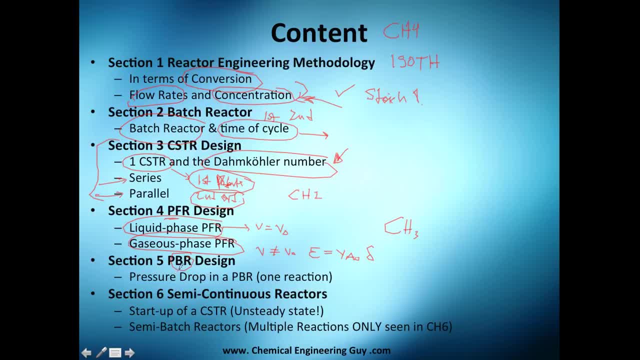 bed reactors. This is the first time we're going to analyze it and we're going to do it essentially for first and second rate orders. We're going to analyze, of course, the drop in pressure, because it's very, very important. Actually, once again, we're going to see only one reaction, because when we go to 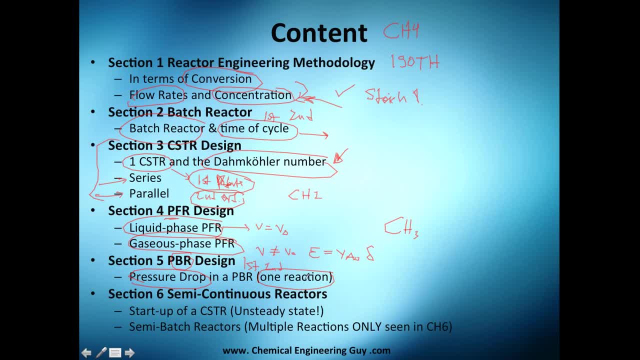 multiple reactions. we're going to use the same methodology for multiple reactions So that if you are willing to see that right now, just go to chapter six and you will see that a PBR with multiple reactions. Now the thing here is pressure drop is calculated by the Ergun or Ergun equation. 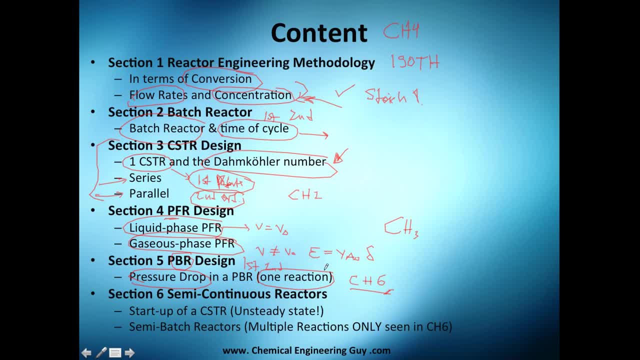 We're going to explain that. It's a little bit theory. Hopefully you've seen it before. in momentum transfers or operations or fluidized beds, all that stuff. It's in the, let's say, in the typical momentum course. You're going to see pressure drops in. 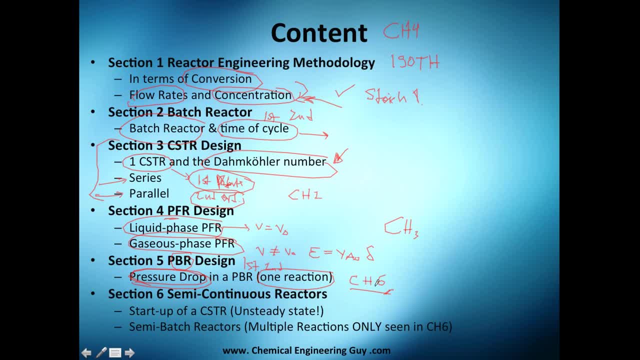 pipes and in beds, fluidized beds, etc. You have no idea. I will make a small overview review. I'm not going to be so specific, so deep in that topic, but yeah, you will at least know what we are talking about. Then we continue with. 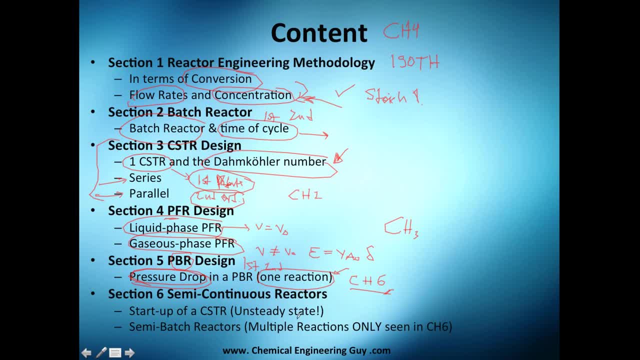 section six, which is semi-continuous reactors. Actually, this one here, semi batch reactor, We're going to see it in chapter six because it's more interesting to see it there, because we're going to apply multiple reactions. A single reaction is not that impressive, so just wait for it. 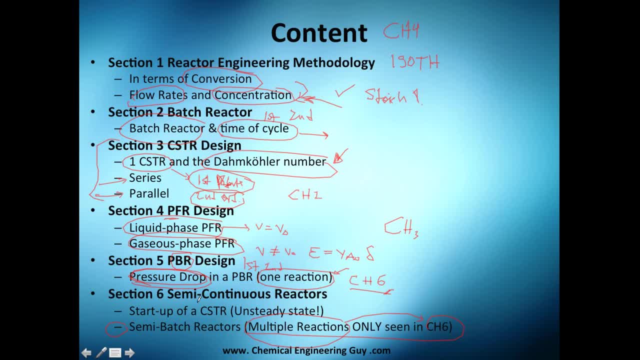 Chapter six is going to come Now. what we are going to see for a semi-continuous reactor is the startup of a CSTR. What does that mean? is that we're going to start our new, or maybe it stopped because electricity go away Or it has maintenance? We have our CSTR and, of course, we need to fill it and we 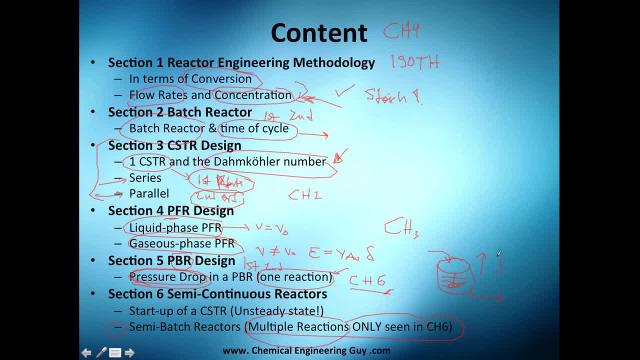 need to react it and we need to increase temperature and levels and all that stuff, And of course, this is in steady state. This is not normal state. We need to be in this state in order to achieve our steady state. We're going to analyze. 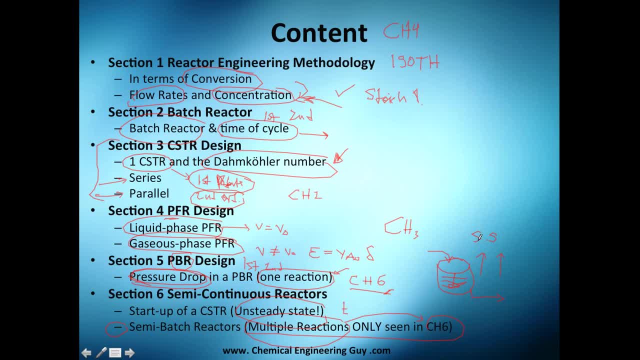 how much time do we need to get to this steady state? And I think it's everything for this video. guys, This was the introduction or overview of this chapter Number four. Next we're going to see section number one, but I'll cut the. 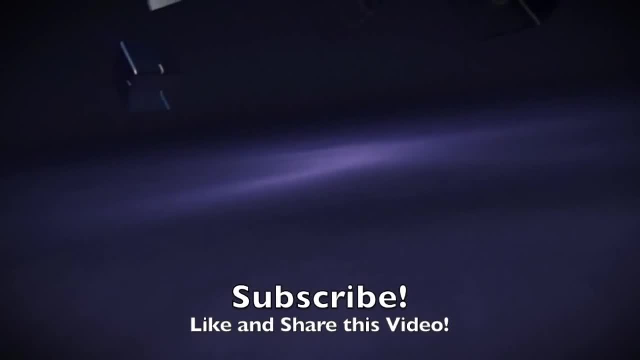 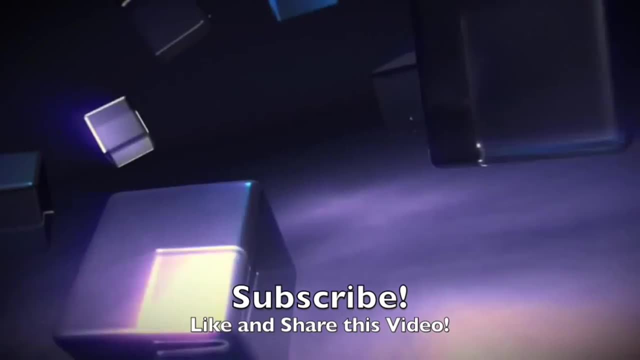 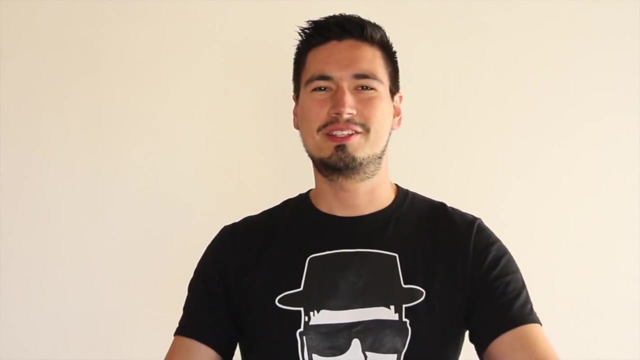 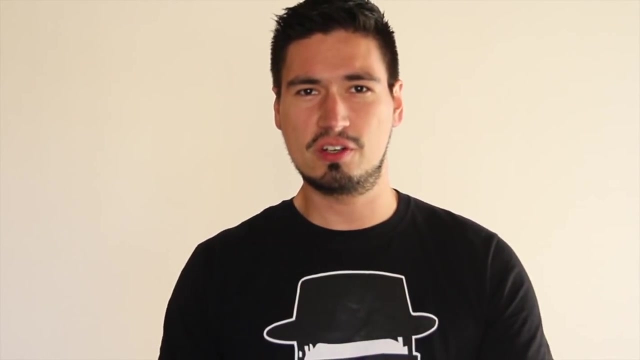 video and see you in the next one. What's up, guys, It's me Chemical Engineering Guy. So if you liked the video, why not push the like button? It really helps me to know if you're liking the videos or if I should be doing more of them. Thanks for watching and I'll see you in the next one. Bye. 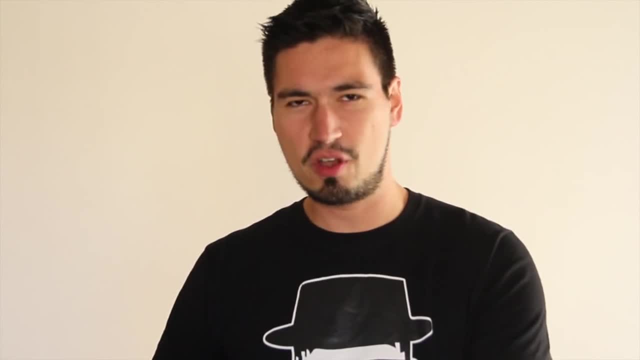 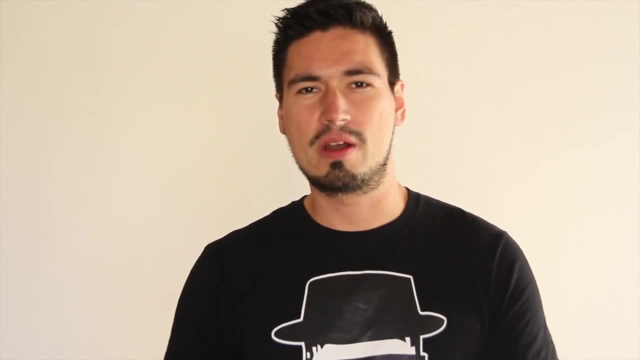 I should be changing something or I should be adding something, taking out content whatever. Also, sharing is caring, So if you got any kind of friends, teachers, colleagues or whatever kind of person that might be interested in this type of content, why not share it? Sharing helps our community to grow faster in. 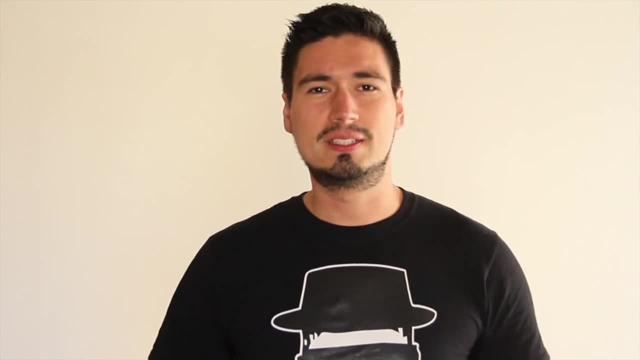 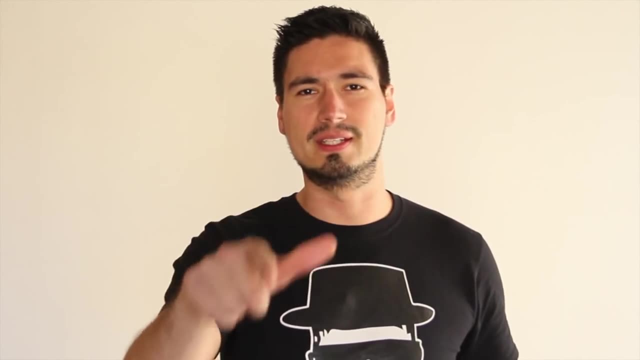 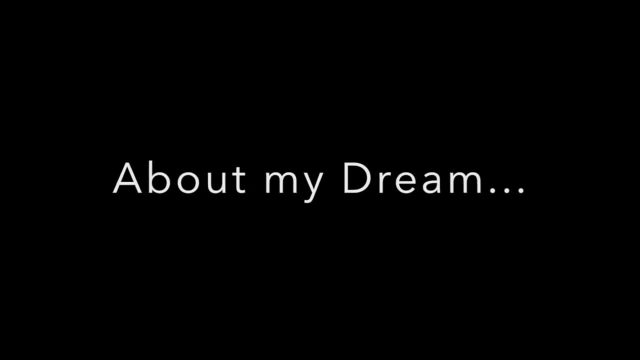 members and in content. If you want to keep track of my activity, videos, uploads, experiments, playlists, whatever content I'm getting in YouTube, be sure to click the subscribe button. Subscribing to the channel is totally free, you guys. My dream is to create an online Academy of Chemical. 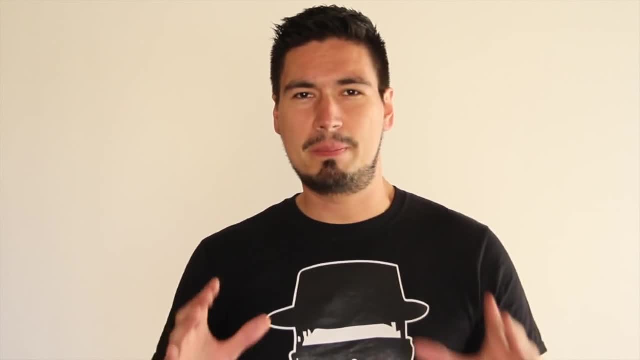 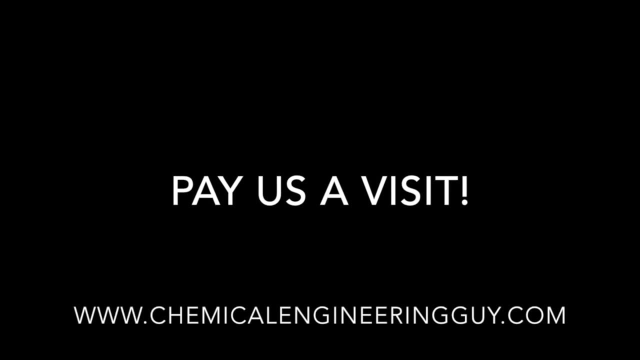 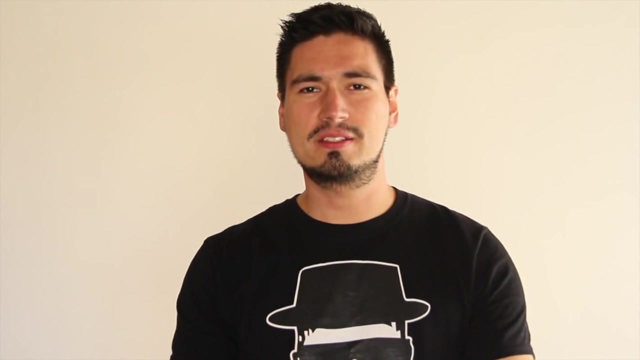 Engineering where everyone can access it in the world. Imagine a place in which the student, the teacher and the engineer get the best of each other. Thank you, thank you, thank you, guys, for the support and the love.